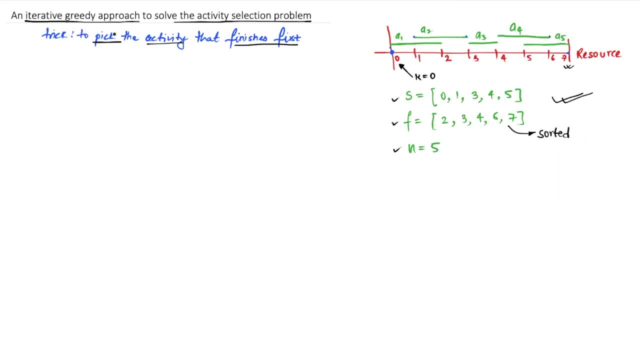 are sorted by their finish times, and the idea is to pick the activity that finishes first. So what we would like to do is implement this algorithm- greedy activity selector- that takes our list of start times and finish times as input, and what this is expected to return is this: set A the maximum size mutually. 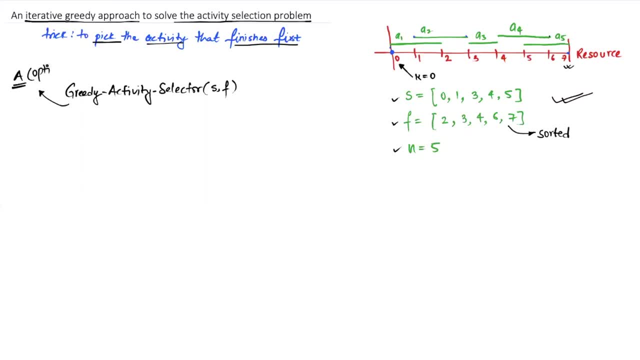 compatible activities, which is our optimal solution. Now let's initialize n to the total number of activities We can do, slength or flength. and then because we know that the activities are sorted by the finish time and that by principle, the first activity is obviously the activity that will be a part of our solution, because they are: 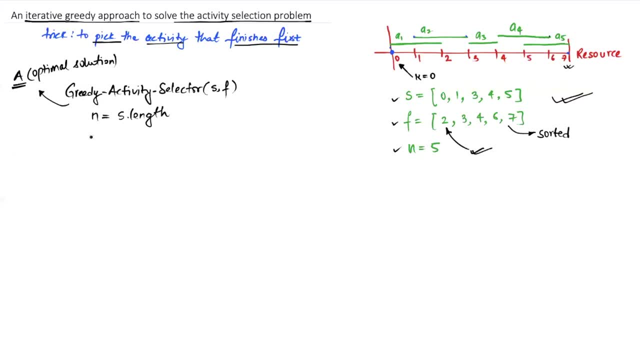 sorted by the finish time, We will pick this activity and put it into the solution. So our solution includes first activity A1.. Now, remember, activity A1 is the first activity based on its finish time, So obviously this becomes the part of the optimal solution. Now what we would like to do is scan. 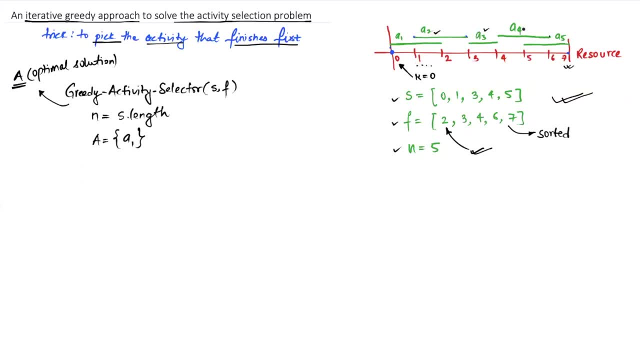 through all the remaining activities, Say, for example, here a2, a3, a4, a5- and then we try to find the next activity by checking the restart times. now we know that the activities are already sorted by their finish times, so all we have to do is throw away. 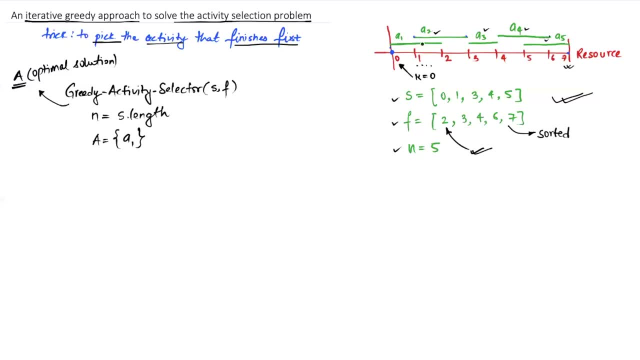 the activities that overlap or are incompatible with our current activity. in other words, if i have a a1 as a part of my optimal solution, all i have to do now is go by the order of this finish time and then keep throwing all the activities that are incompatible with a1 as long as i throw all. 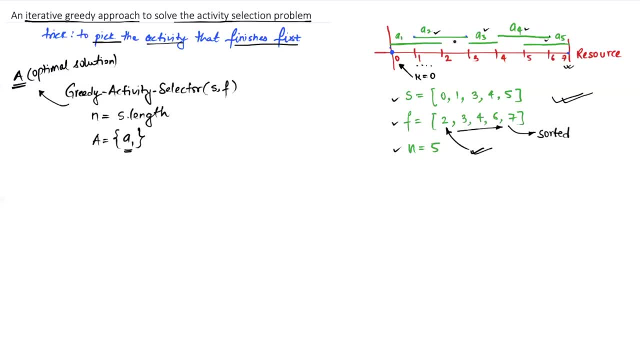 the activities that are incompatible with a1. the next activity that's compatible with a1 will be a part of the optimal solution, because they're already sorted by the finish time. now, to represent our most recent activity added to the optimal solution, i'm going to use a. 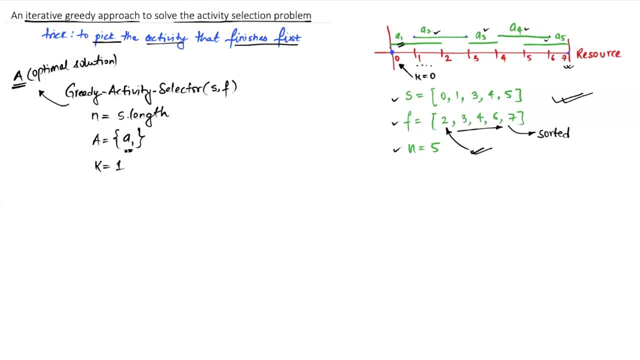 this index k to represent this. because a1 is the most recent activity added to the optimal solution, i will use this index k to represent most recently added activity to the solution. so i'm going to scan all the activities, starting from the next activity to the nth activity, and check if the 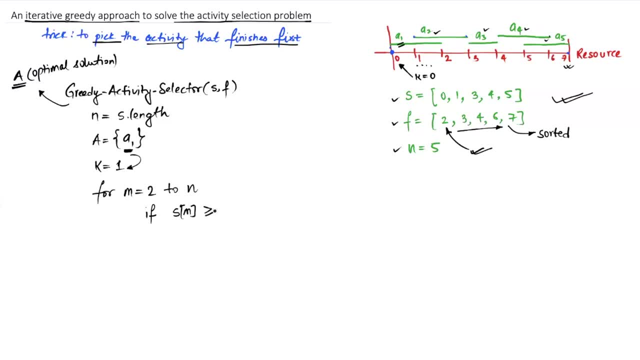 start time of this activity m is more than or equal to the finish time of our current activity. so here a2's start time is not more than or equal to the start time of our current activity a1. so that means that we have a start time of a1 which is more than or equal to the finish time of 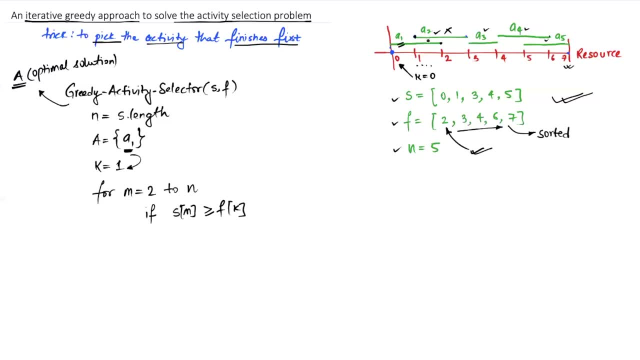 a1, so we do not want this activity. this is incompatible. if this happens, then we will keep looping through. otherwise, if we find an activity whose start time is more than or equal to the finish time of our previous activity- so this is a and let's say this is m- then we will add this to. 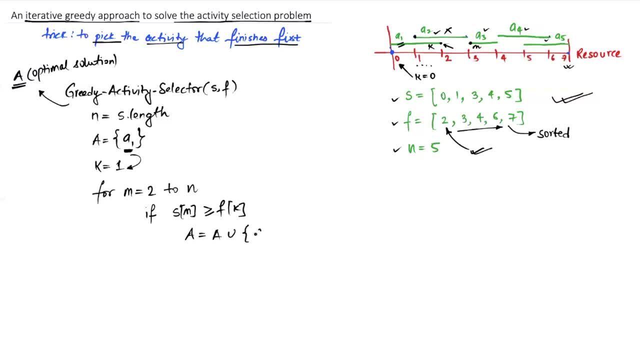 the part of our optimal solution. so if this happens, then we do a equals a union. we add now am to the. do this, we set k equals m, so that now our current solution, m, becomes the previous solution. or in other words, now we mark this activity a3 as our k, so that we start looking at the finish time of a3. 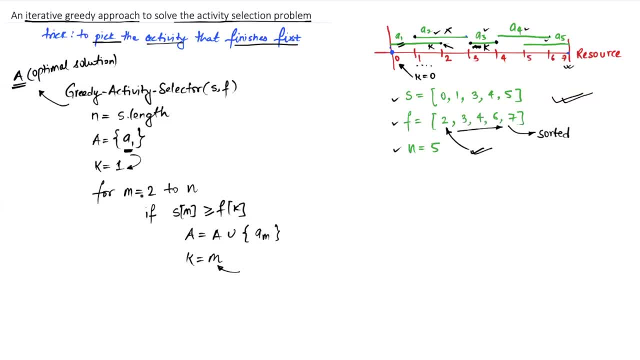 instead of a1. and then, finally, once all of this is done, once m runs from 2 to all the way through n, we simply return a, which is the set of the optimal activities. now let me trace this algorithm one more time to further clarify the flow. so we have s and f as input. we have n equals to 5, our optimal. 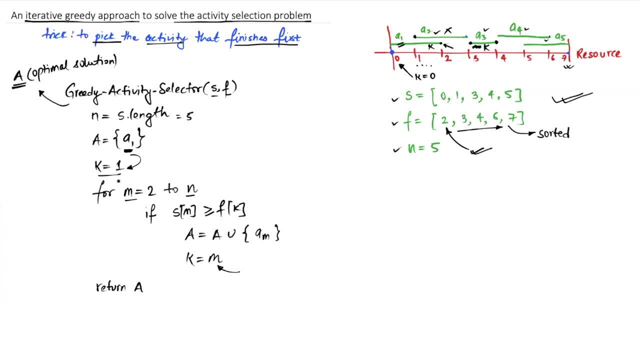 solution includes a1 and then we have k equals 1, so we start from m equals 2 through n if s2- so we check- is s2. that is s for activity number 2 more than or equals to finish time for activity number 1. so start time of the second activity is: 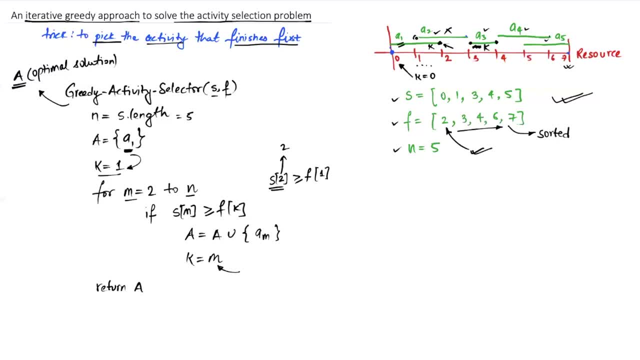 1 and finish time of the first activity is 2. so a start time of second activity is not more than finish time of first activity or is not even equal. so this is incompatible. so that means this: if your statement executes to false, that means we continue through the next item. we have m equals 3. now then 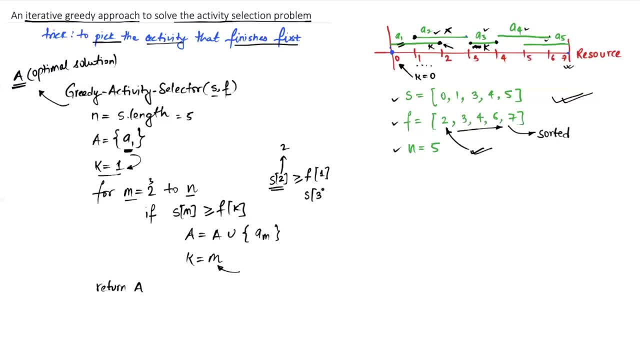 we check, is the start time of this activity 3 more than or equals to the finish time of activity 1. so does it mean for us if we start t3 or if we don't start t3? the medications vary from t3anten to t4. this is often the case. so when we say start m equals 4, it means that now. 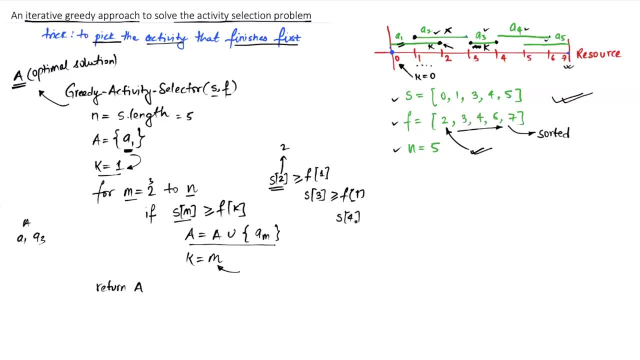 r is a infinite of 0.06 on xh of sum now ready. its relate to aO here as well and we see if start m equalsO at t3 is equal to m, or rather if, let's say, if the activity has more than or equals to finish time of activity 3. only once is we check if the start time of activity 3, which is 3 more than or equals to the finish time of a1. this is true. so now we add a3 to the solution. so our a now initially had a1, now it has a 3 as well. and then we set k equals m. next we increase m to 4. so we check: is start time of activity number 4. 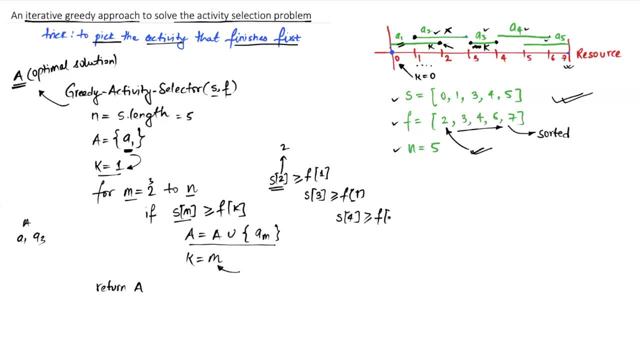 more than equals to finish time. now K is already three. finish time of activity number three. so we are checking: is the start time of activity number four greater than equals to the finish time of activity number three? this is true. so this means we add a four to the solution, so a four becomes a part of the optimal. 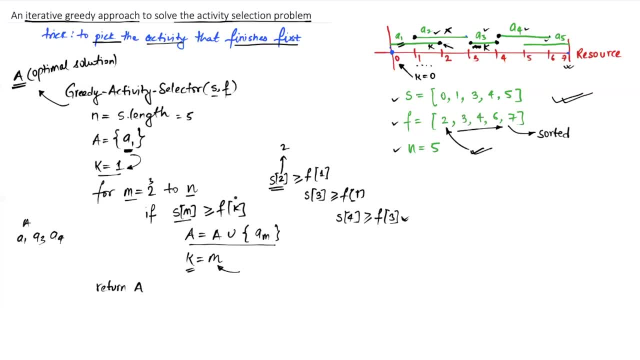 solution. and then we set K equals to four, so then we have K equals to four. we have M equals to five. now we check: is s5 is start time of activity number five more than or equals to the finish time of activity number four. so start time of. 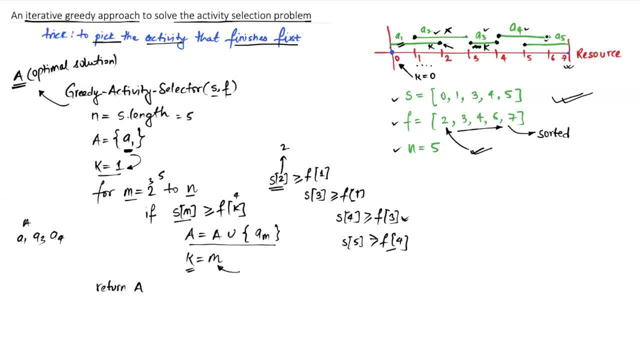 activity number five is five and finish time of famine. number four: it's six, so s5 is not more than f4, and so we do not run this part. and then we end the for loop and we finally return a 1, a 3, a, 4: this 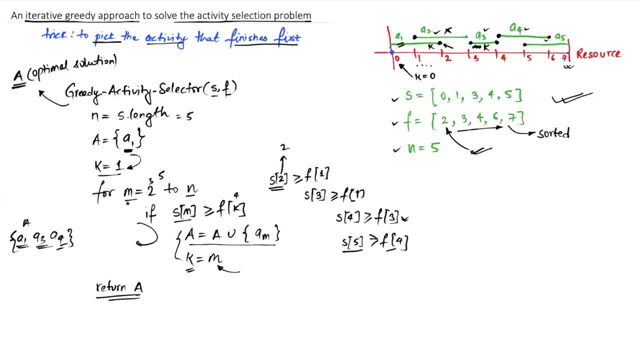 set and this a ENDS our optimal solution now, because we scan all the activities once. the running time of this algorithm is big theta of n, where n is the number of activities. now remember this running time assumes that the activities are sorted by the finish time. if they are not sorted by the finish time, then the running time of